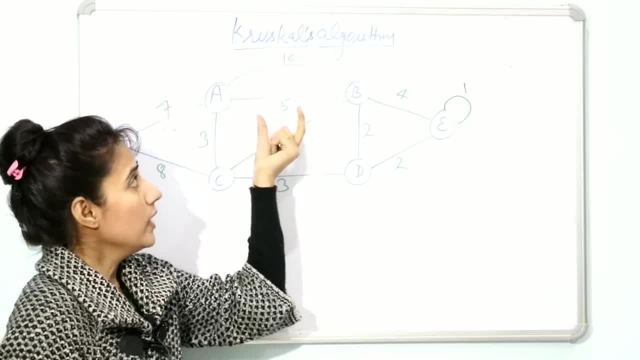 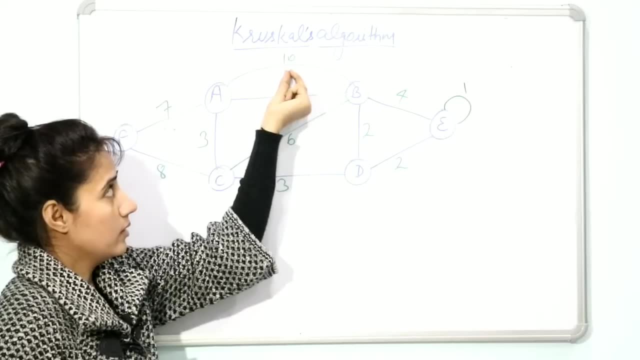 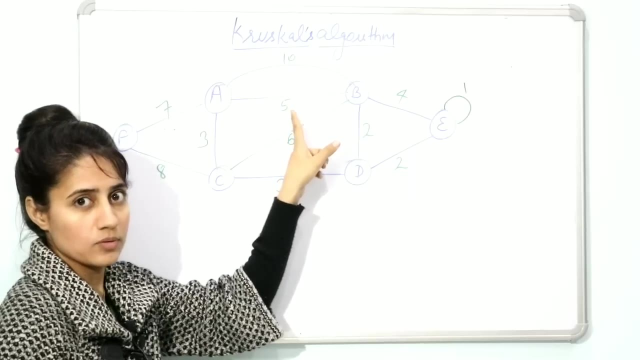 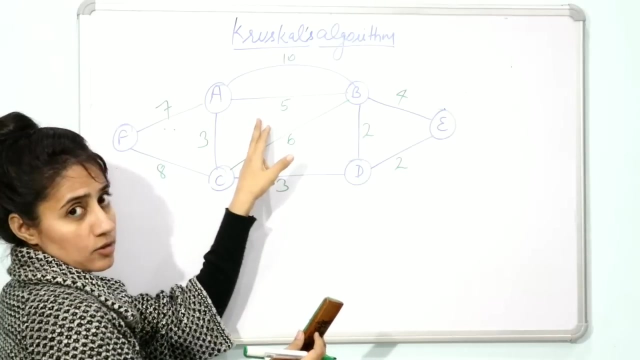 have How to delete. You will keep that edge having minimum weight from five and ten. Which one is having minimum weight, Five? So you will remove this ten and you will keep this five. Okay, So first step is remove all the loops, Loops we have deleted and parallel edges. Parallel edges means I have shown you how to delete Minimum edge weight. 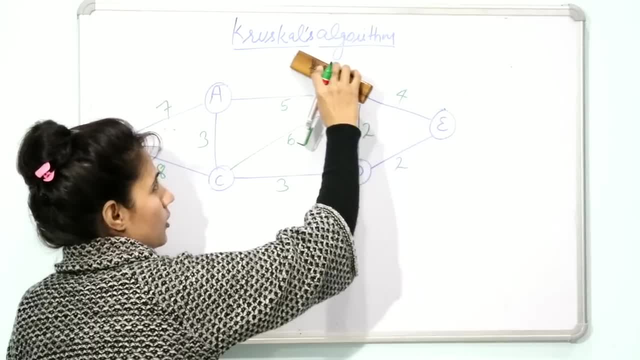 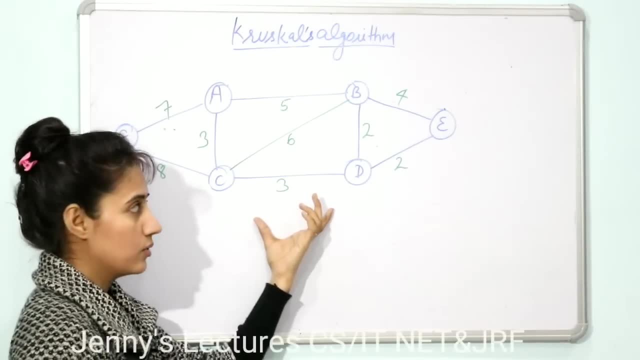 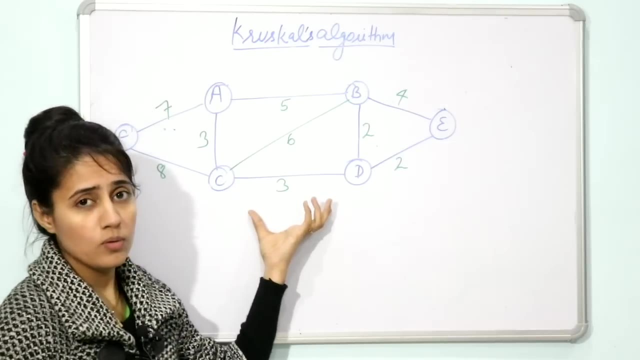 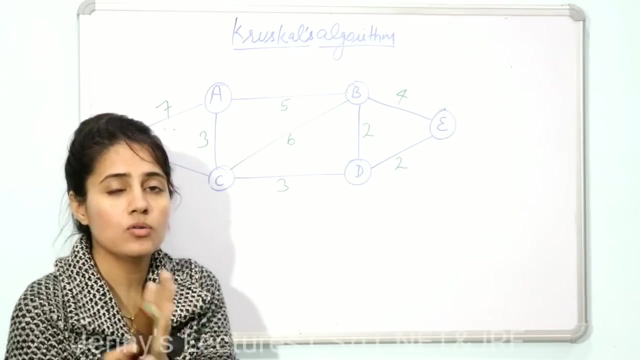 you will keep that one and maximum, you will remove that one. okay, so after first step, this one is our graph. now what is the next step? in cruscal algo, you will arrange all the edges according to their edge weight, and in which order? in increasing order of their edge weight. okay. 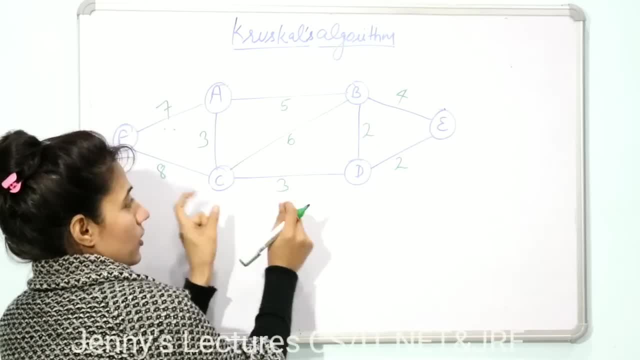 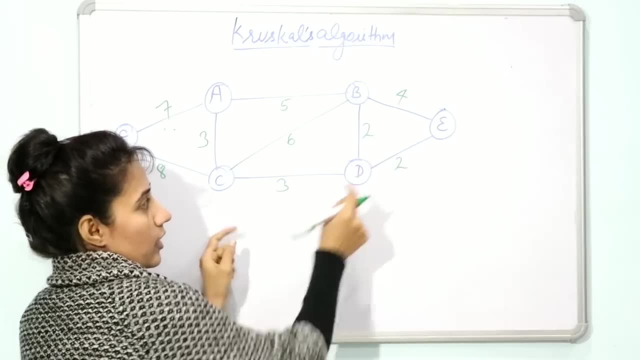 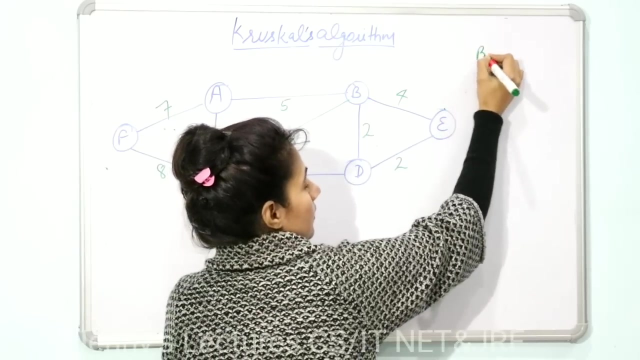 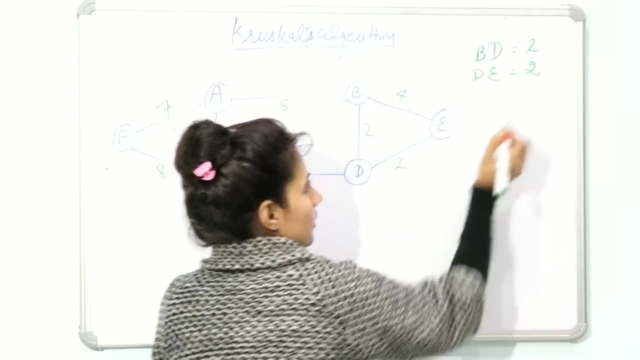 now see increasing order of minimum edge weight like cost or cooking weight minimum. it is 2, two and two. we have two edges having their weight so you can write all the edges first of all, if suppose we write BD having edge weight 2 and then DE having edge weight 2, 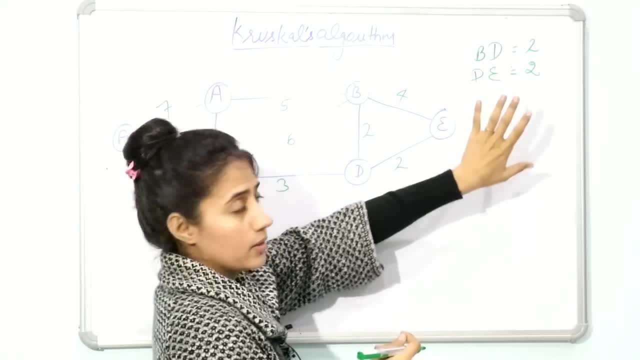 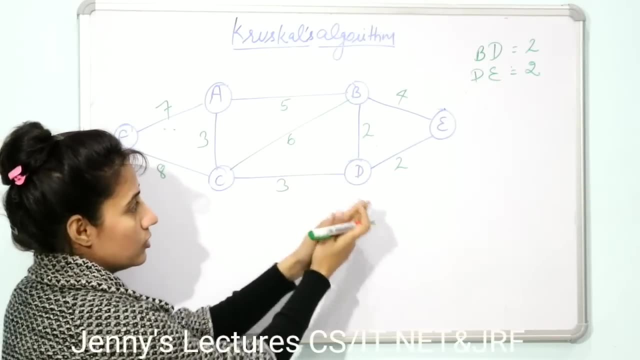 see. first you can write DE or BD. well, it is not matter. fine, 2 and 2 is minimum. and that week they came 50 kgędämäÄÄôs paid mm 빠�i sampý' 2. now next minimum weight is you are supposed to write in increasing order: 2. 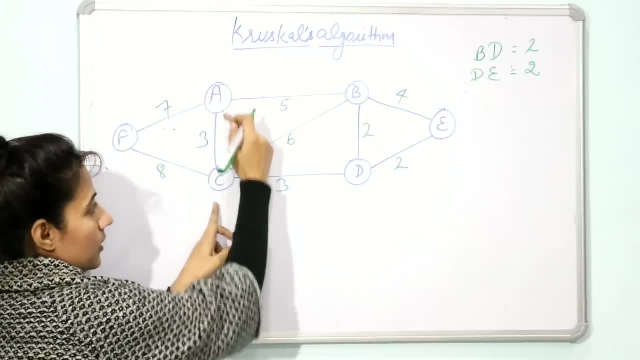 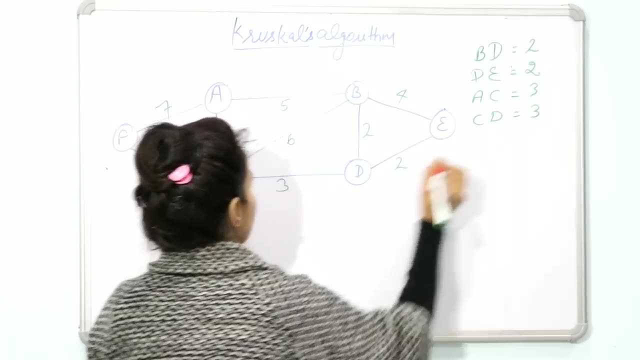 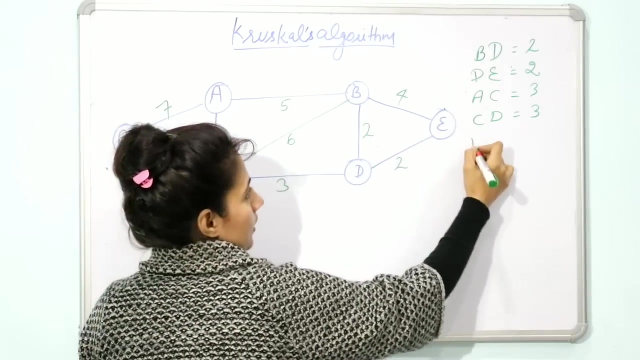 ke baad apne paas kya hai. 3, 3 ke bhi. we have two edges, AC and CD, so you can write AC and CD having 3 and 3, AC and CD, fine now. next we have this 4, 4, hem hamare paas kya hai. b he is having edge weight for fine. next, Apne paas fore. 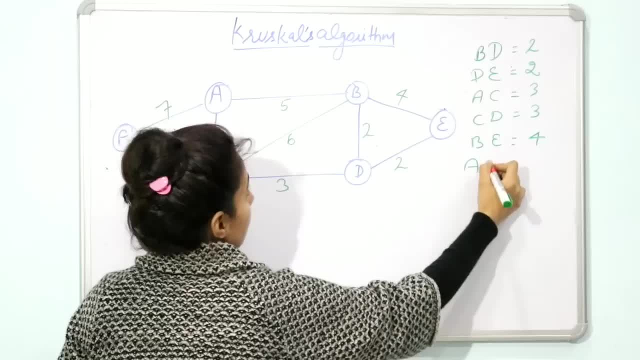 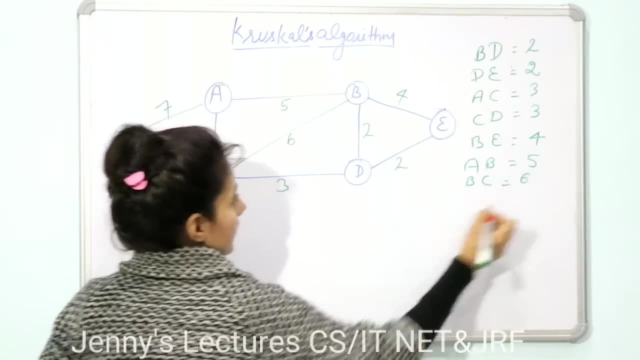 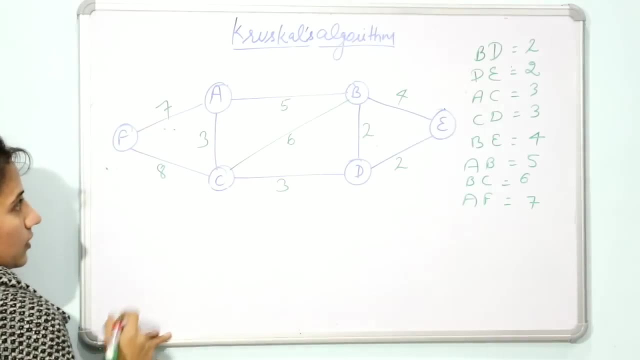 ke baad. kya aega. this one, 5 AB A B is having edge weight. 5. next is this: 6 b C is having edge weight. 6. next is 7 a F is having weight 7 and 7 k. baad we have one left, that is fc is havingổi. 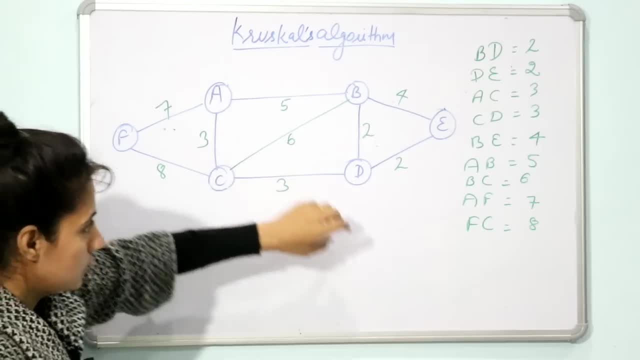 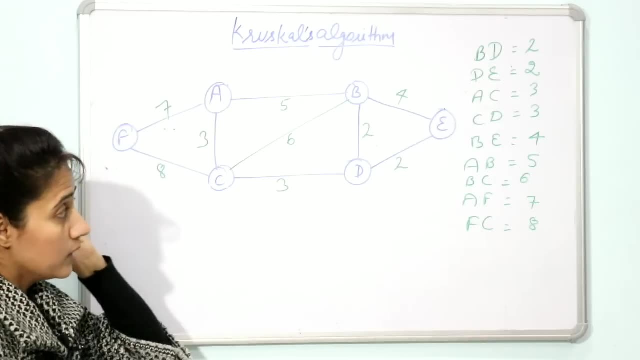 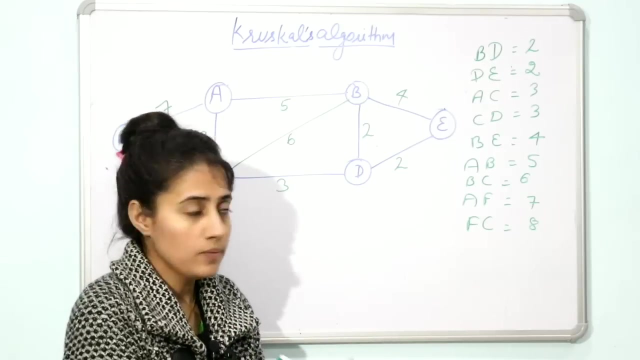 Ko. Yeah, boys, My, no one want another one. actually, she is always getting her head edge weight 8, I hope all the edges. we have written all the edges in this. okay, then see next step. you are supposed to write down all the edges in their increasing edge weight. fine, now third step is what you will choose. the 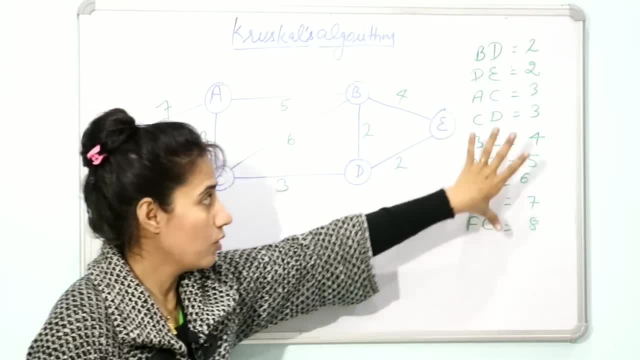 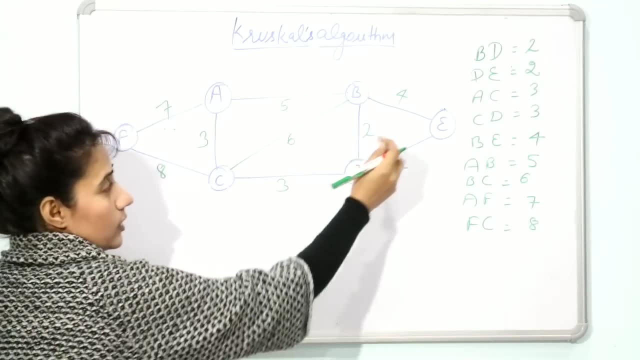 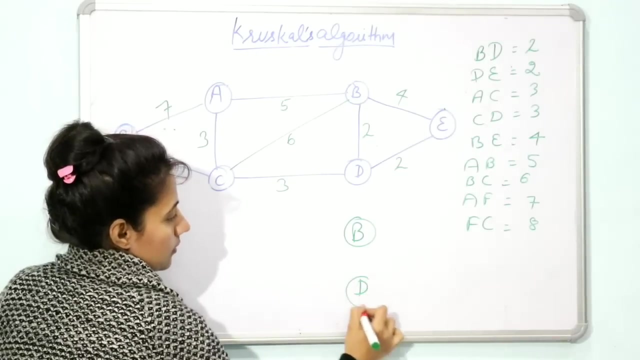 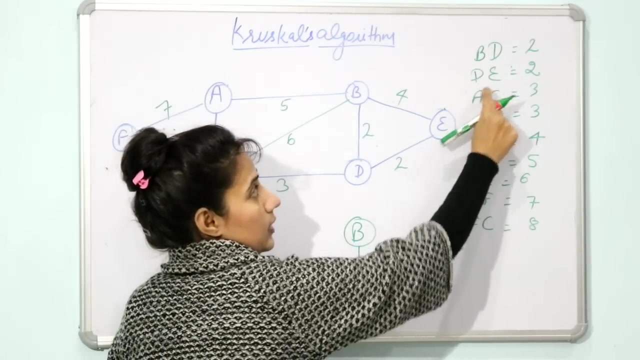 edge, having minimum edge weight from this set. fine, okay, now the first is 2, then you will choose this one: B, D, B and D having edge weight. what 2 this you have chosen next is what D, E you will choose and you will connect these edges. 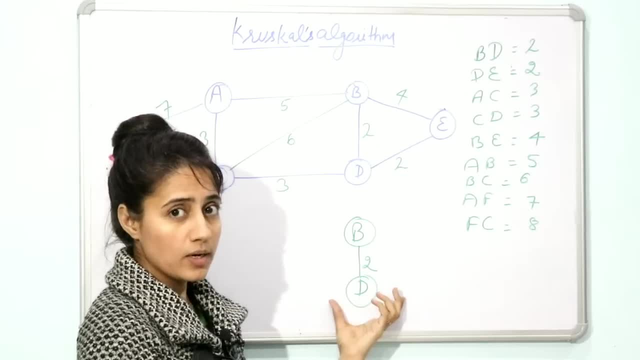 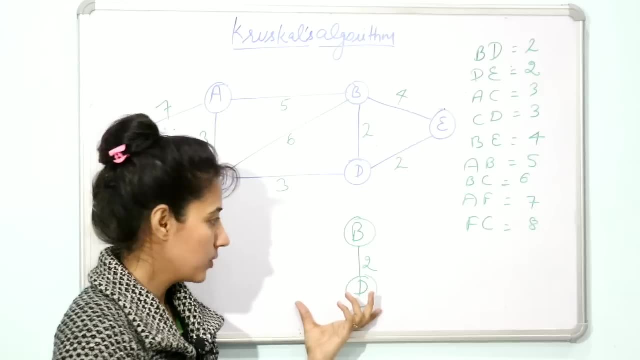 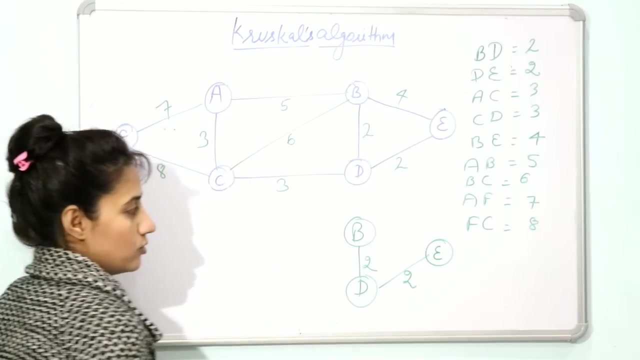 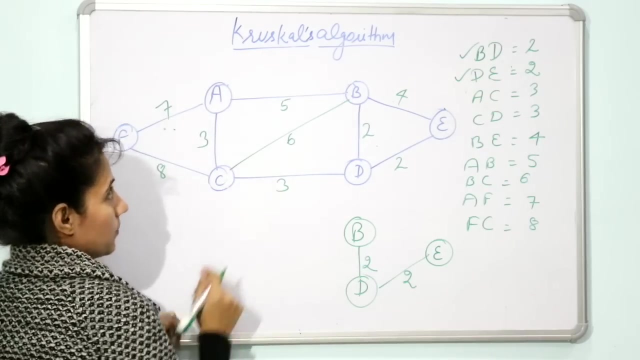 that it is fine. while connecting, you have to take care it should not contain that mst which you are forming. it should not contain any cycle. fine, next time discuss. the next is D, E, D and E. it also contains edge weight. it is also having edge weight. 2. fine, this one is done. this one is in now. next is AC, AC- you. can connect with AC and then sweetness, having Minecraft also, but it's, according to us, can connectester- is coming only in Central America, where when you have c, it is a field called Gaudiya. it is below that c and it that's corresponding to frank. you can connect this also. we have escrever ставl, but it will provide. 301 class that you can connect the time to D and D and E. two words: are you able to read the? with respect, it is 25A Protech964. that is on income arra directly neatly flashing curve. all the tables are appropriate. connect com if you want to write C, which is C about 5 against H, resisting Twitch by. 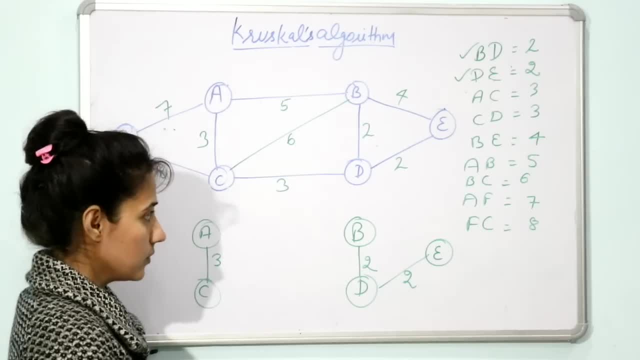 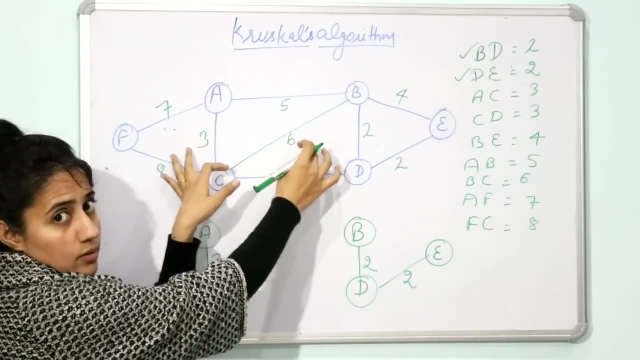 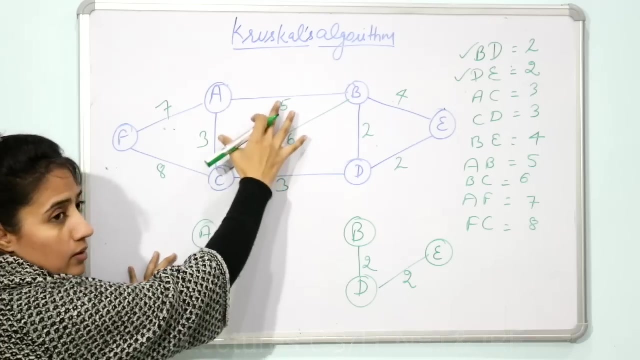 edge weight having 3. fine, see, it's not compulsory that you will write it like this. I am just writing in this manner because I have a graph like this, so you know to understand it better. I am writing it like this as it is written in my given graph. next is AC. that is also. 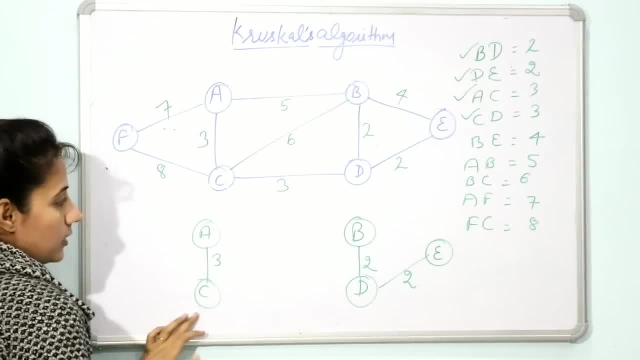 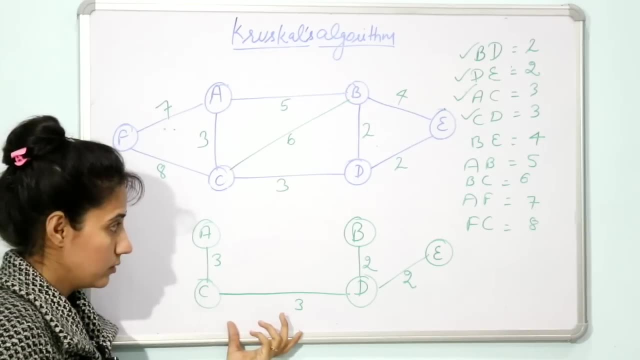 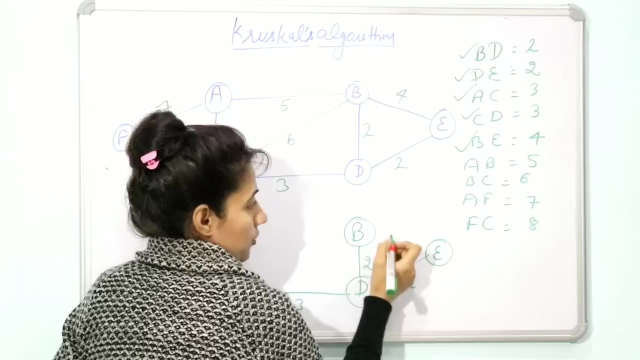 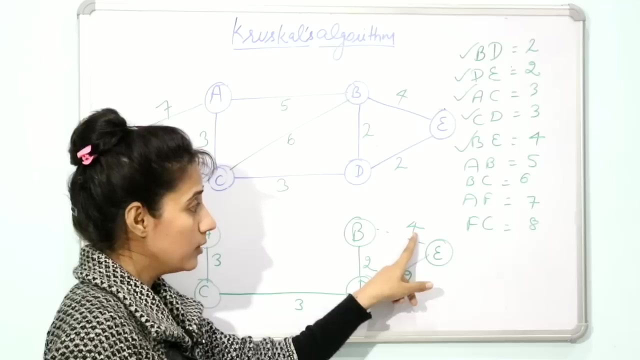 done now. next is CD C and D. obviously you can connect this one because connect kardiya and it does not contain any cycle. fine, so you can connect it. next is BE. next is BE that is having 4, BE 4. but you cannot connect this one, although it is having minimum weight, see. 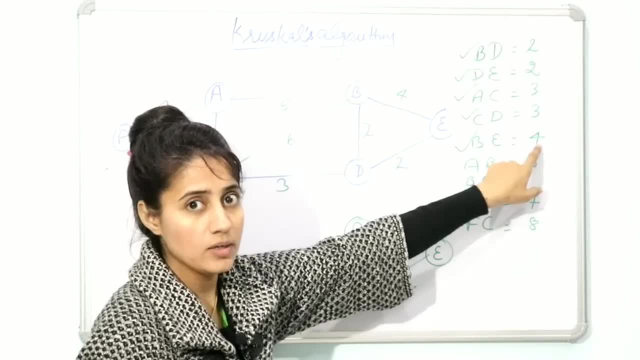 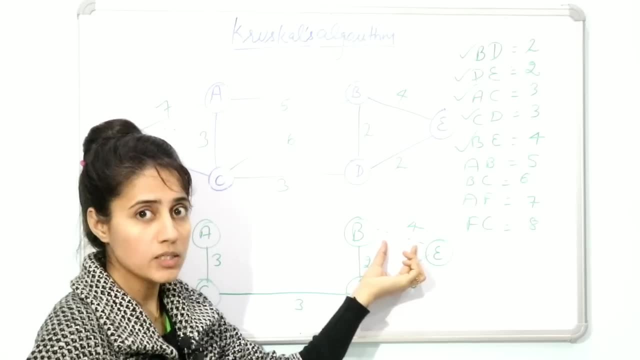 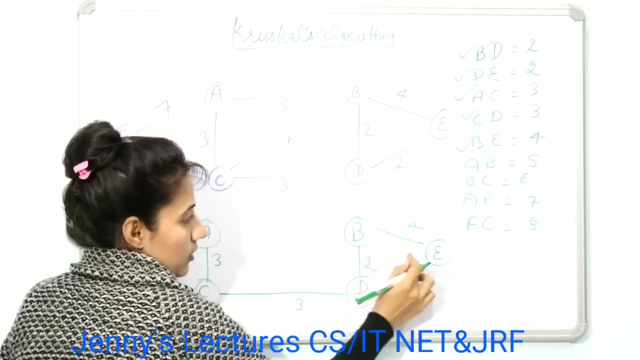 weight is less than 5,, 6,, 7,, 8. ok, and our funda is this: only that minimum weight is minimum weight. we have to take that edge, but you cannot connect it. see, one more condition is there. you cannot connect it. why so? because as soon as you connect it, it will form a cycle. 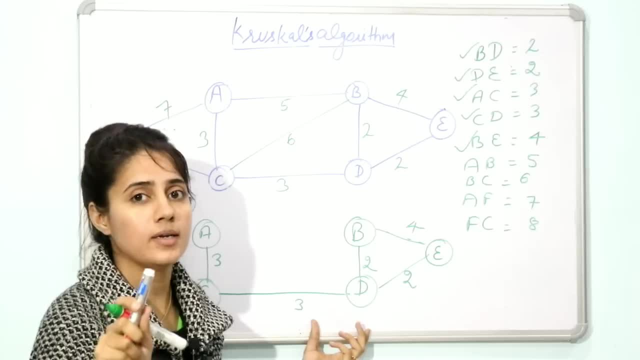 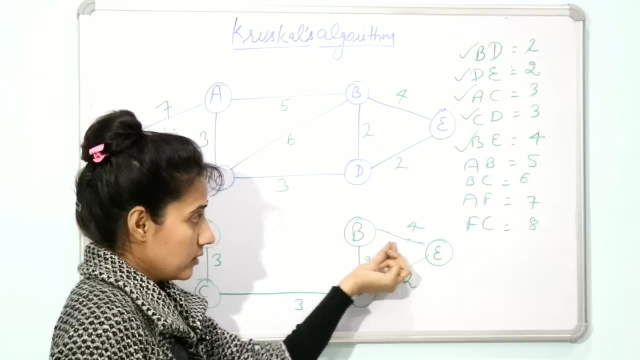 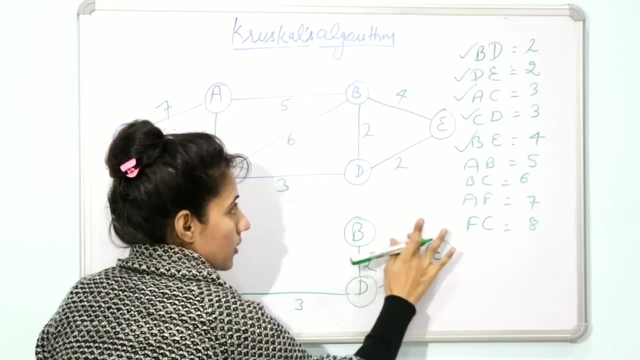 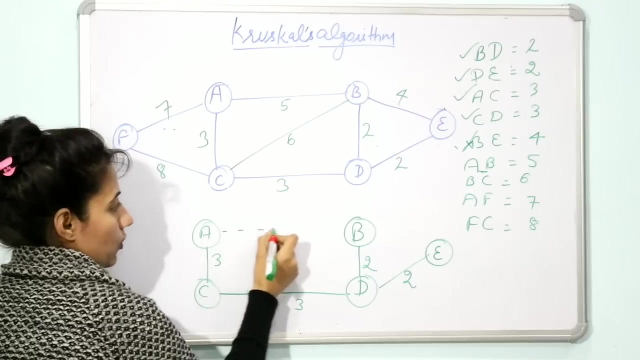 fine, and one of the property of MST is that it does not contain any cycle. fine, so you cannot- you know form- or connect that edge which results in a cycle in MST. ok, so you cannot connect it, so we will leave this one, fine. next is AB. now can you connect AB? no, 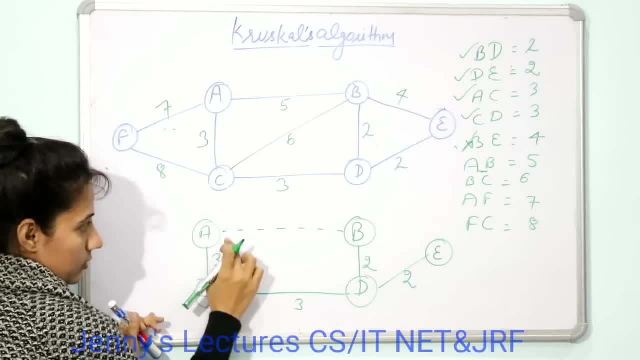 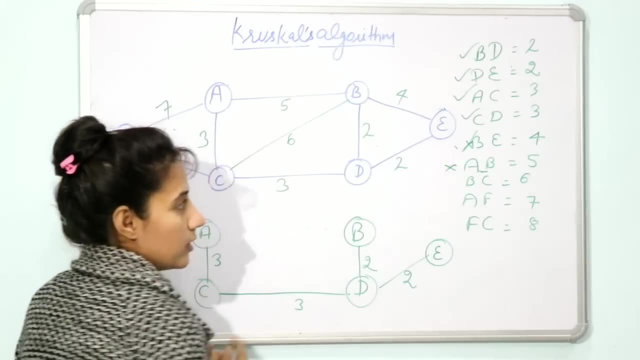 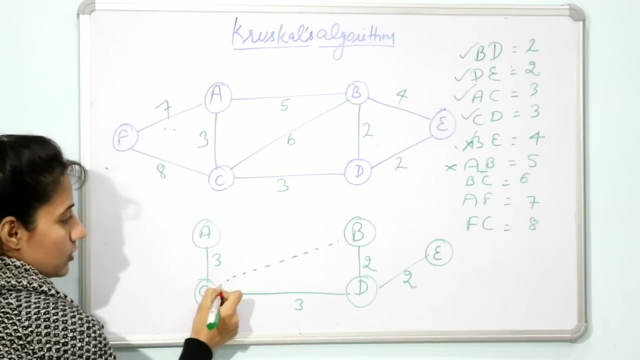 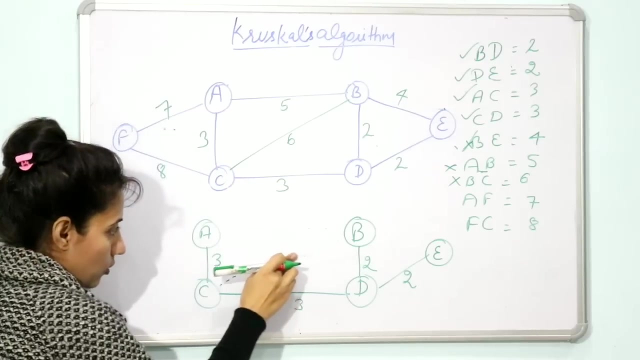 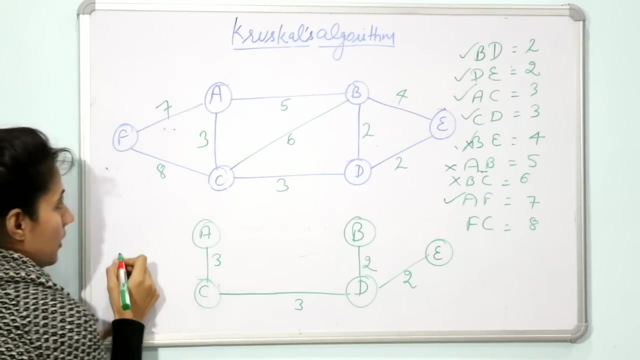 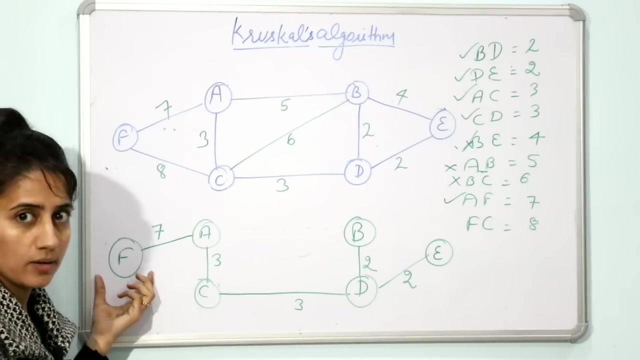 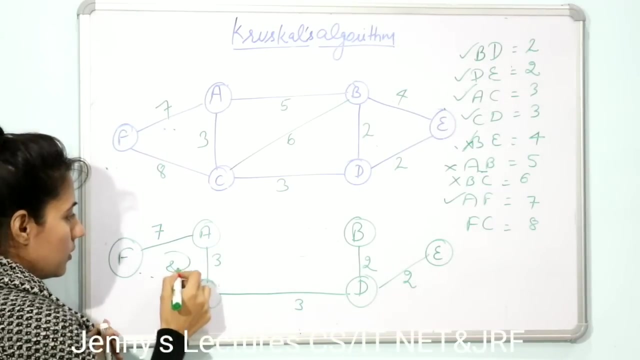 you cannot connect because this also will form a cycle and MST does not contain any cycle, so you cannot connect this. also, you cannot connect this. also, you cannot take this. next is BC. can you connect this one? can you use this? H, B, C? no, because it also contains a cycle, so you will leave this. also, you will not take this. you cannot connect B and C. next is AF. can you take this one? yes, you can take AF, because when you will connect A to F, then it does not form any cycle. fine, connected. next is FC. can you connect FC? no, it will form a cycle, okay. 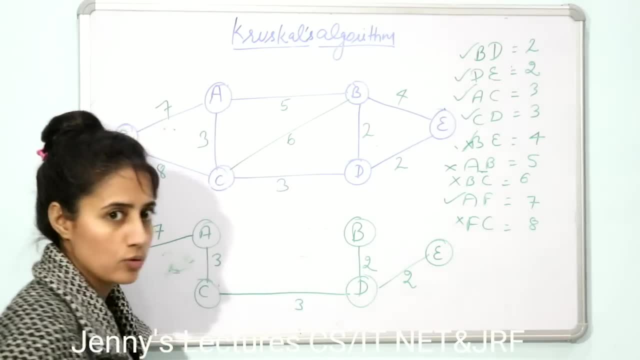 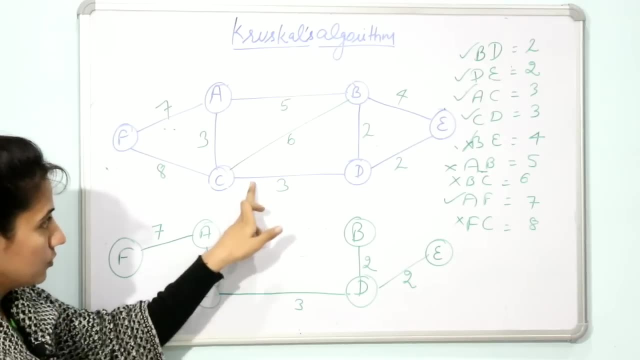 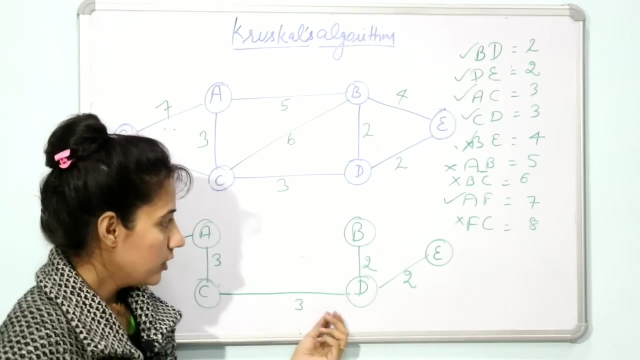 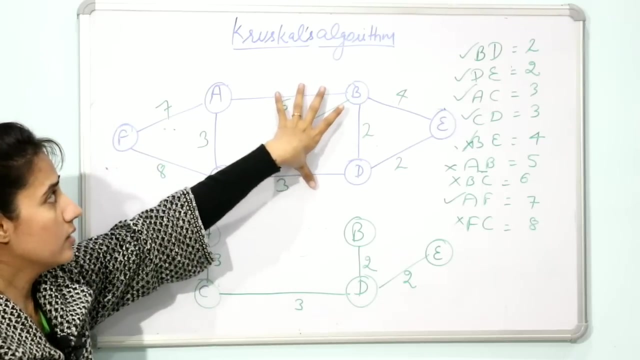 so leave this one also and we have, you know, no other edge left. so this is the minimum spanning tree of this graph using Kruskal's algorithm. fine, see one property I have already told you, that is MST, does not contain any cycle. second property is: what if that graph, given graph, is having n number of vertices?